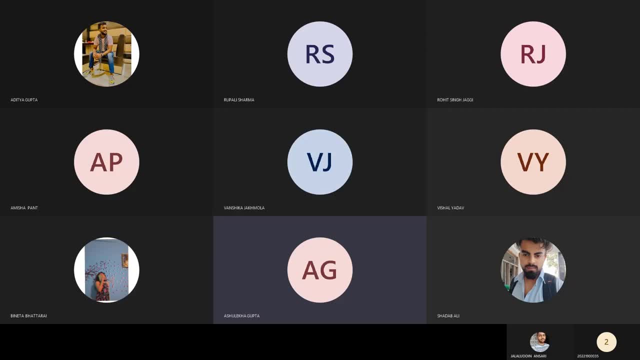 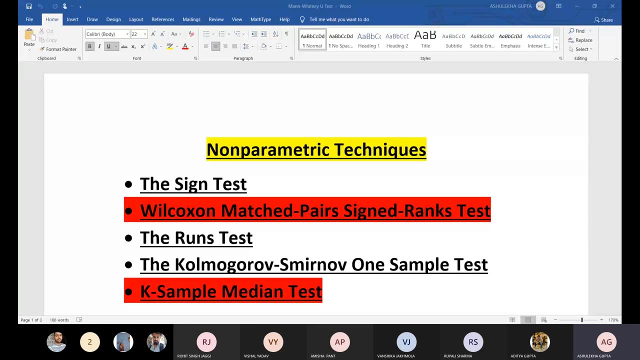 We are going to start nonparametric techniques, right, Nonparametric techniques. Do you understand by term nonparametric techniques? Because I had already explained you when we are going to start parametric test and when we are going to, when we are, when we are doing nonparametric. 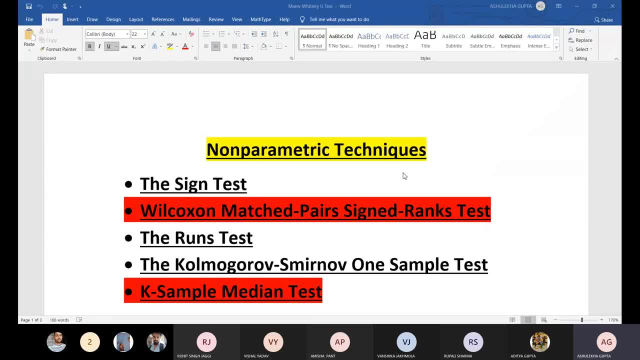 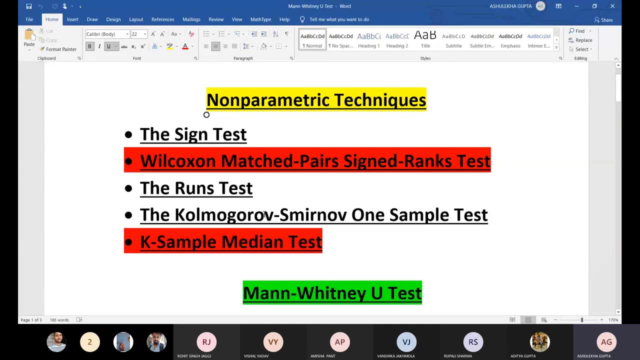 test right. So in the nonparametric techniques there are the some options to nonparametric techniques. we are using The sign test right, Wilcoxon, mesh pair sign rank test, the run test, Koglow, Kolmogorov, Semironov- one sample test, K sample median test. So today, 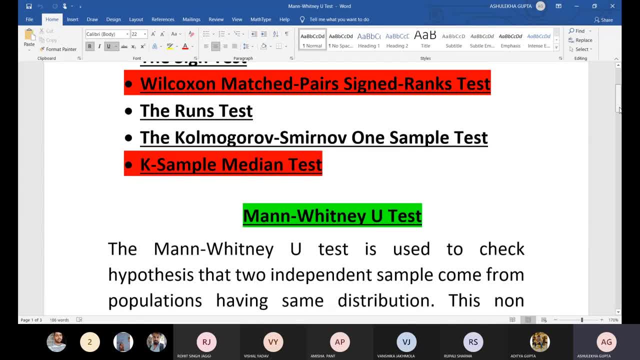 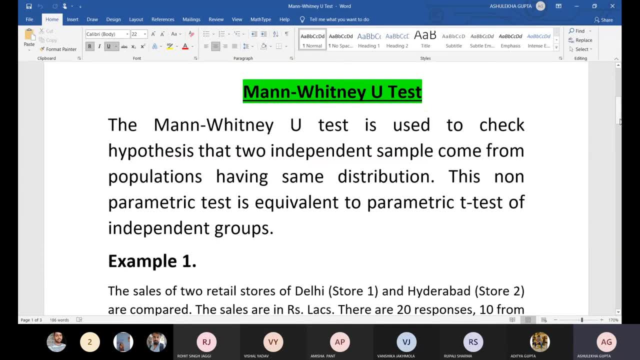 now we will start. we will work on Mann-Whitney U test, right? So basically, first of all, we should know what do you mean by Mann-Whitney U test. Hota kya hai, Toh? Mann-Whitney U test is used to check hypothesis that two independent sample. 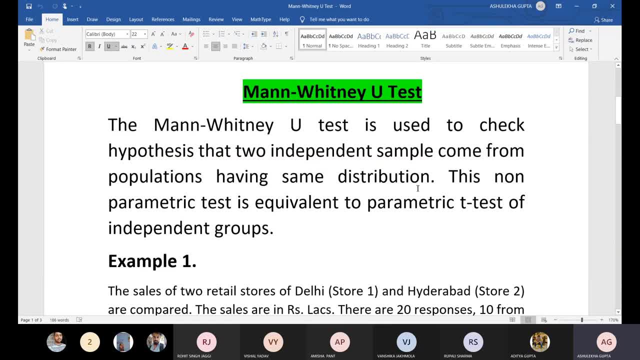 come from populations having the same distribution hai na Aapko yaad hoga. jab maine aapko T test kar aaya tha, toh T test. it is similar to T test. Hamne jahan ek baar independent. 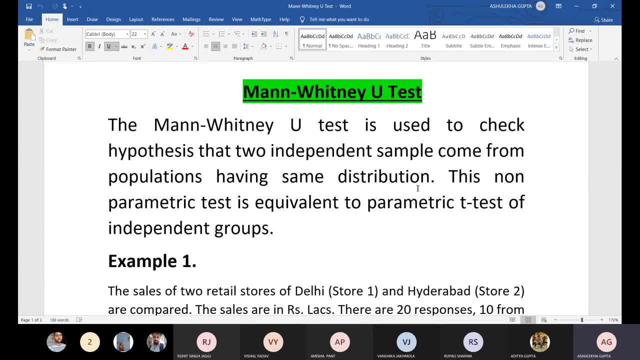 T test lagaya tha, or ek baar pure T test lagaya tha. So it is the independent T test. So yaha, par dono sample independent hai from each other. right? Come from populations having the same distribution, but two different, two independent samples, right? So this nonparametric 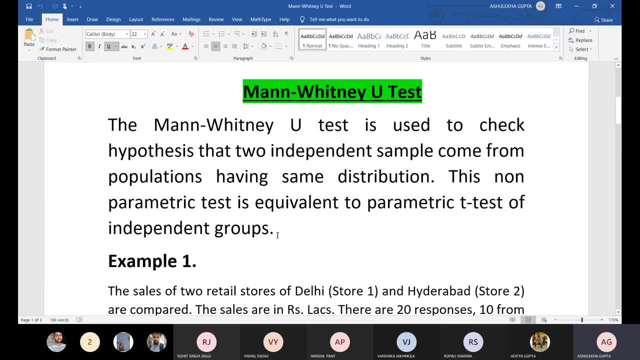 test is equivalent to parametric T test of the independent groups. It is a very similar kyunki, because wo parametric tha isliye hamne T test lagaya wapa ye nonparametric hai isliye hamne Mann-Whitney U test, yaha par hum apply kar rahe hain. Ab let's say I am taking. 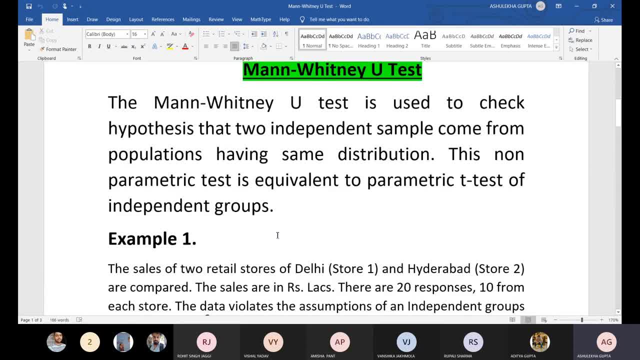 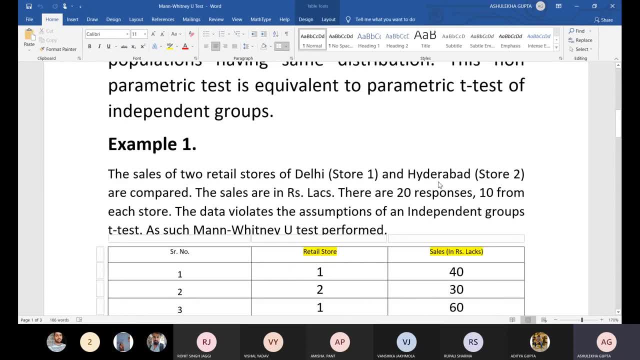 one example. it is a very simple example: two sales of two retail stores, of Delhi, store one, and Hyderabad Do metro cities hai ek metro ko hum dusse metro se compare kar rahe hai retail stores hai right Hum unki sales ko compare karna chahte hain right Sales. 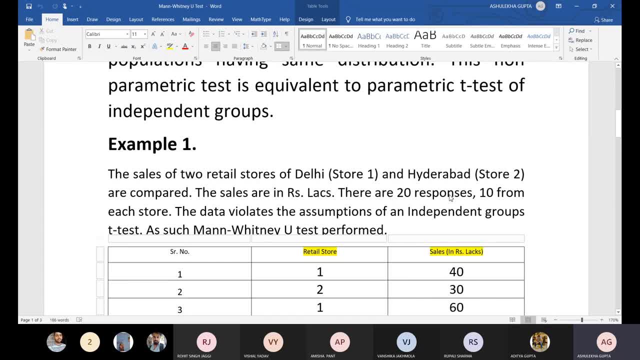 kisne hai are in rupees lakhs. So there are 20 responses. we had collected humne 20 response liye hain, 10 from each store, 10 humne Delhi ke store se liye hain 10 humne. 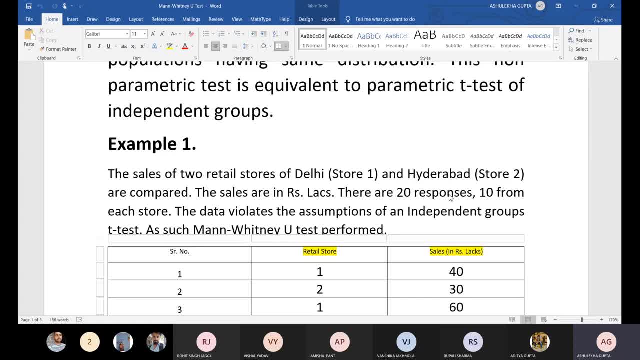 Hyderabad ke store se liye hain right. So data violates the assumptions of the independent groups. T test, SH Mann-Whitney U test performed right Kyunki data. humane ye kehar raha hai. humane assumption: ye kehar raha hai ki there is no difference right In the sales of both. 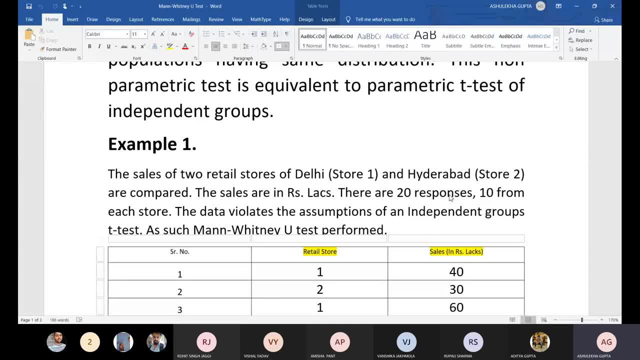 these retail stores Delhi and Hyderabad. that means, we can say, this is our hypothesis Ab now: we will either accept or reject right Delhi or Hyderabad ke retail stores, so kyunki stores ki sales mein koi difference nahi hai. they are saying: right now, humne jo data collect kiya. 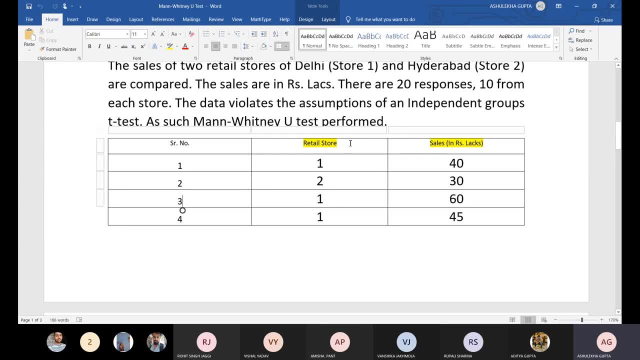 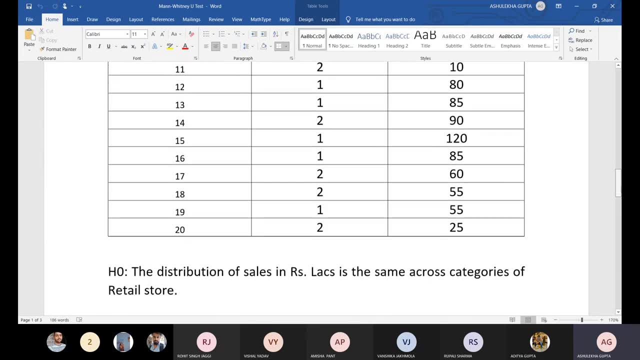 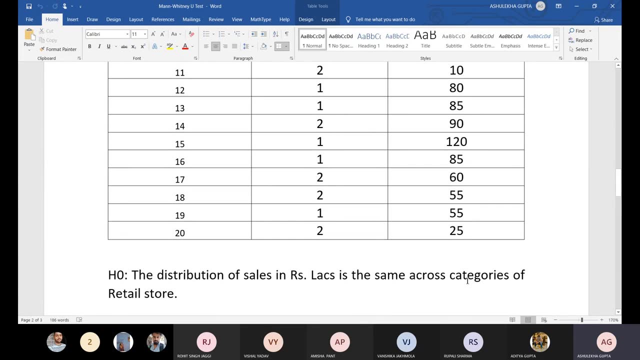 hai. we have taken right teen column hai yaha par serial numbers retail store and sales in the rupees lakhs: right 20 respondents ka data is here. right 20 respondents ka data is here. this is a null hypothesis. the distribution of sales in rupees lakhs is the same across categories of. 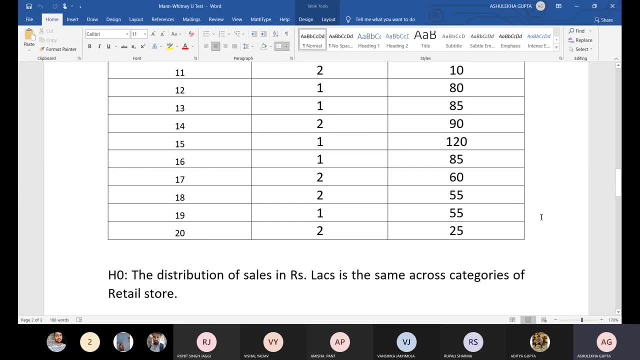 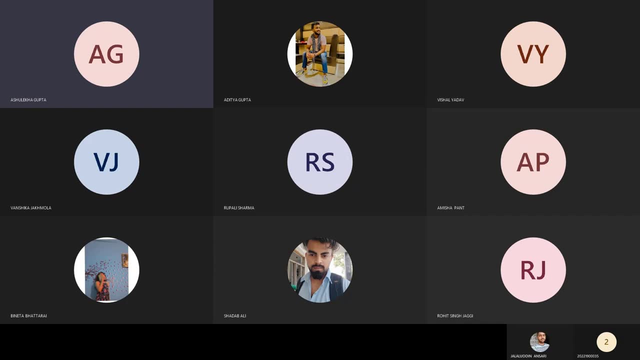 the retail store right. so now what i have to do now i will share with you my sbss file. correct, and in the sbss file you could see here in this sbss file, this is the non-parametric test. right in this non-parametric test you could see here: 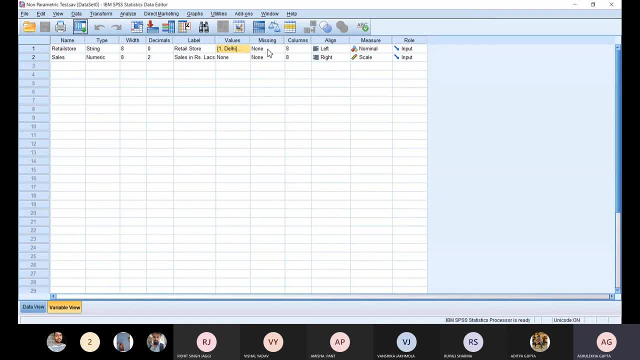 i want two columns. mujhe do columns se right. maine in do columns say: ko yaha par define kar diya. first variable hai mera retail store. that would be string. string hoga right or nominal hoga ye right retail store. nominal hoga kyunki ki either one number or two number. 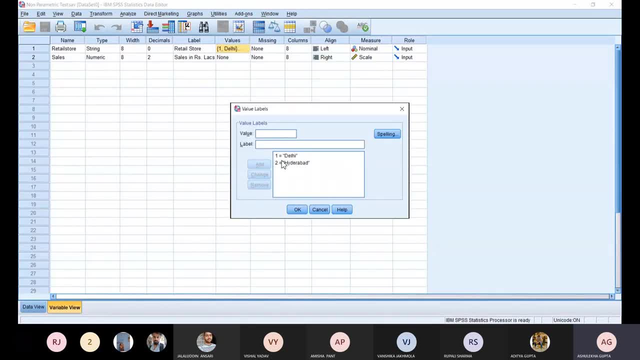 yaha, maine define kar diya retail store me. one maine kaha delhi ke liye, two maine kaha hyderabad ke liye. right, i have defined. and then sales, agar hum jaate hain, right, sales we have. we said ki that would be sales in the rupees lakhs. 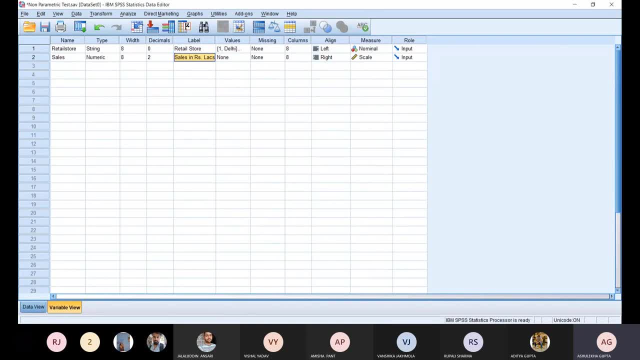 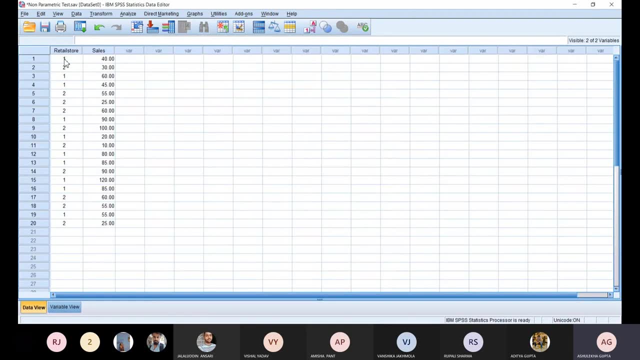 do decimal point tak mujhe chahiye. that would again a scale. now we can see data view, data view me. aap dekho, mujhe do column mil gaye, aur is data, ko maine apni word file se yaha copy kar liye. 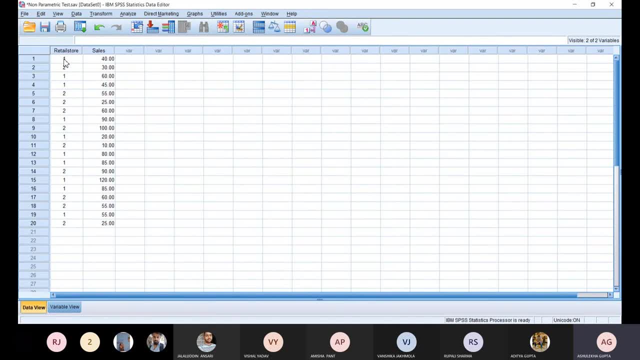 to that means we understood. one means delhi, two means hyderabad. right ab, hum run karenge test, hum analyze me gaye. we went to analyze humne dekha yaha se. agar aap dekhe one, two, three, four, five, six, seven, eight, nine, ten, eleven, twelve, thirteen, fourteen, fifteen, fifteen. 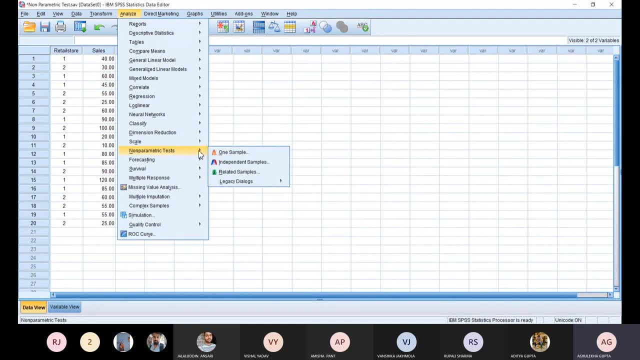 eleven, thirteen, thirty three, ninety seven, ninety three, ninety seven, ninety seven, thirty eight. Ath nabar pe nonparametric testers. he hai right non parametric test me humara sample, chuki related sample. nahi hai right humara sample, kya hai? that is our sample? 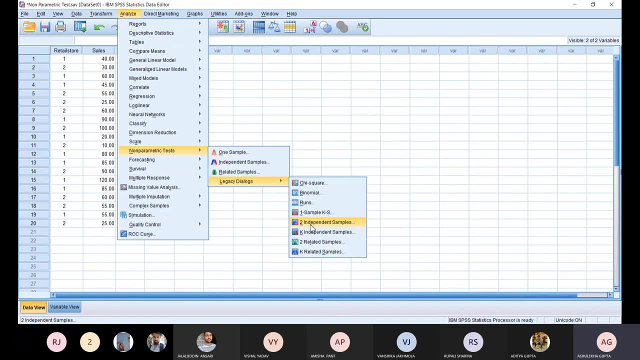 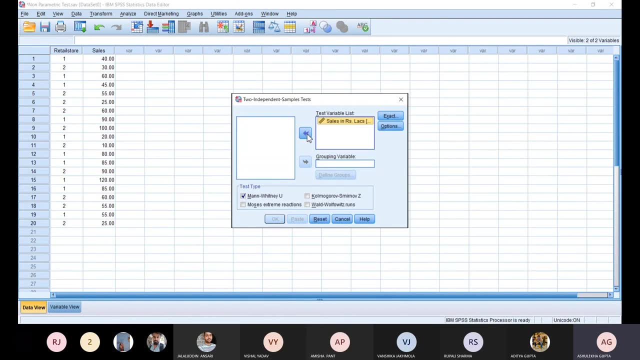 is two independent sample right hum kaha jaenge. two independent sample pe. two independent sample pe humne click kya. now you could see here: right, sales hai sales ko humne test variable me dal diya. and what about the group? you can see here point to point number. so how many? 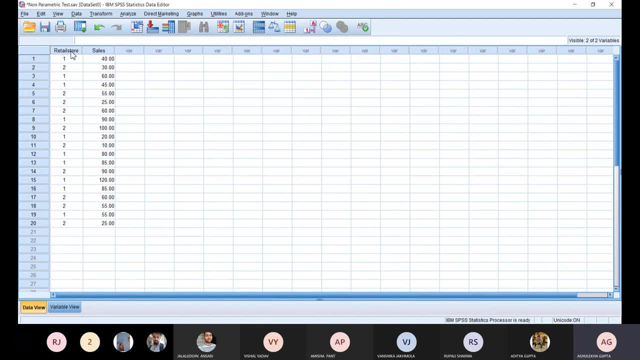 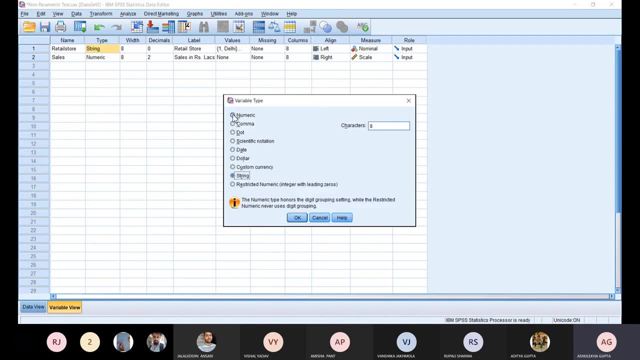 just a moment, group variable. actually, what we have to do, we will take numeric and we will take scale also right, numeric. and here is: we will take scale correct. we have done a small correction right now, again, what we have to do in data. you see, here we will go. 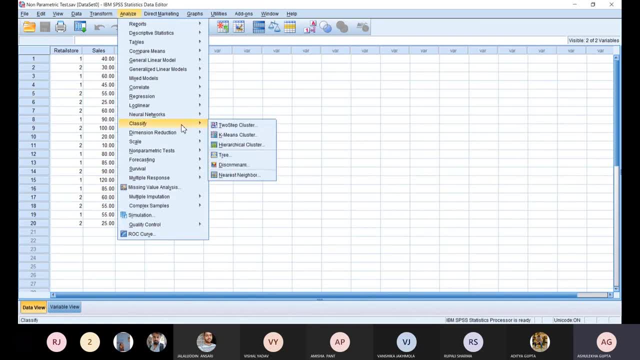 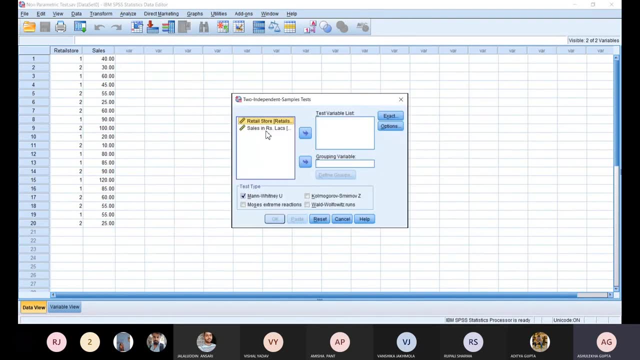 to analyze. we will go to non parametric test. right then, we will go to independent sample test. now you could see here: sales are test variable and retail. what will happen? our group variable will happen. now we will define groups here one and there is group 2 is 2, 1 means 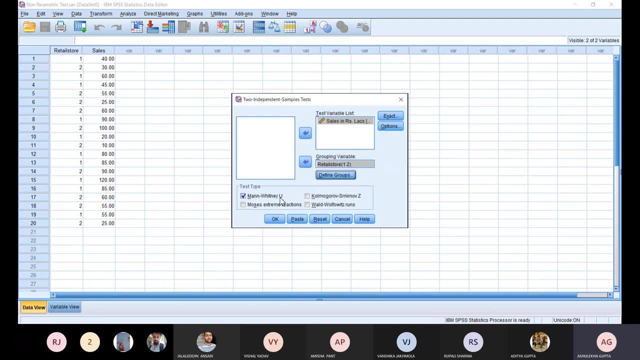 Delhi 2 means Hyderabad. we have ticked here, but we have not done the test yet we have. We don't want to test Colmar Grove, we don't want to test Moses Extreme, we don't want to test Waldwolf. what we want is simply this test: Manvayati test. 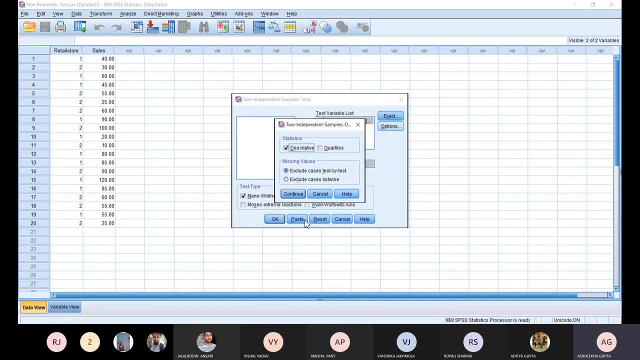 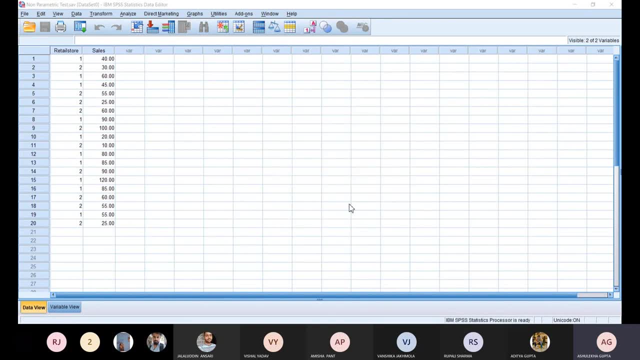 And if we also want descriptives, then we will tick on descriptives. we will continue this, right? So we press on OK, right. So now you could see here. I will show you the option. this one is the output file I am going to share with you. I am going to share with you output file. 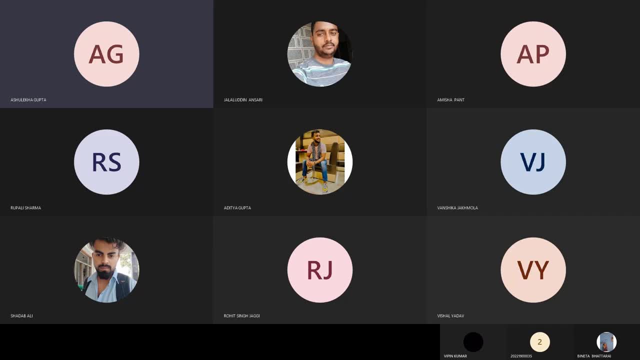 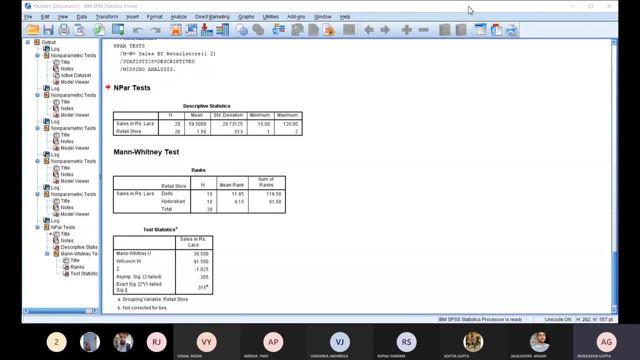 Right, you could see here. this is my output file. right in output file. you could see here in output file. we can see here: there are: these are the descriptive statistics, right? these are the Manvayati test, right? I have 20 sample right mean values, standard deviation, minimum, maximum, minimum value, maximum value. 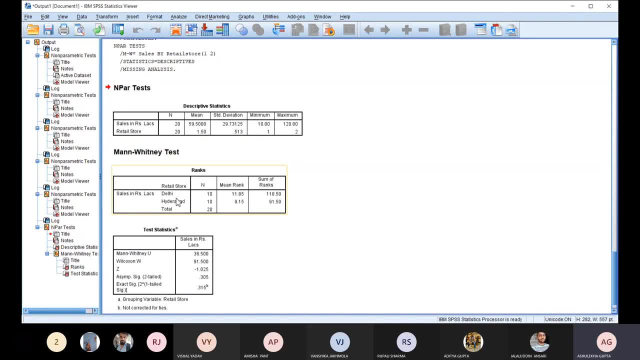 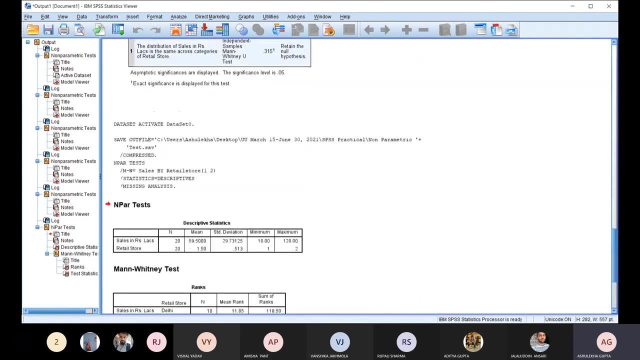 In Manvayati test you will see same Sales in rupees. Delhi has 10 cases. Hyderabad has 10 cases. their mean rank has come. sum of the ranks has come. Now, you could see here. you could see here, right, we could see here. this is the. these are the. this is the non-parametric test, right? 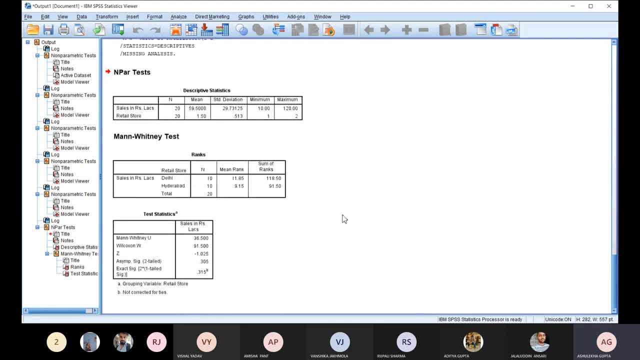 Now you will see in non-parametric test. here you can see this is the and sales in the rupees. Lex right Manvayati test 36, right. Wilcoxon W91, Z. test has come right. assumptions have come. this one is the assumptions. significance at the two table is 0.305 and exact is 0.35, right. 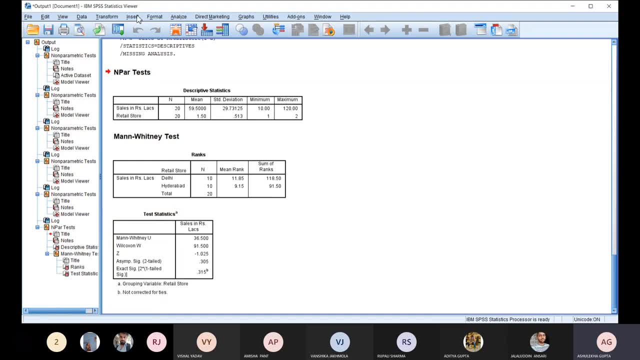 Now you can see we can do one more thing in this. again. we will go to, again, we will go to analyze. we will go to analyze, right, If we go to analyze in non-parametric test and we ticked on independent sample, right? 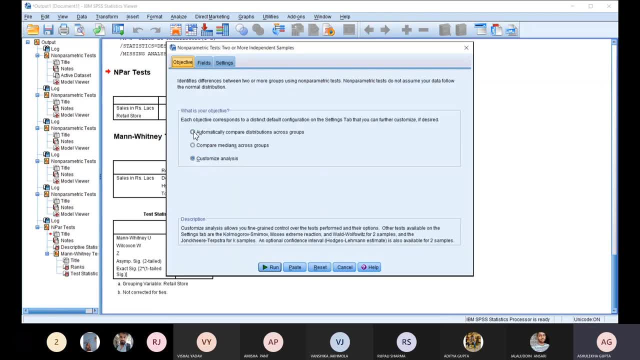 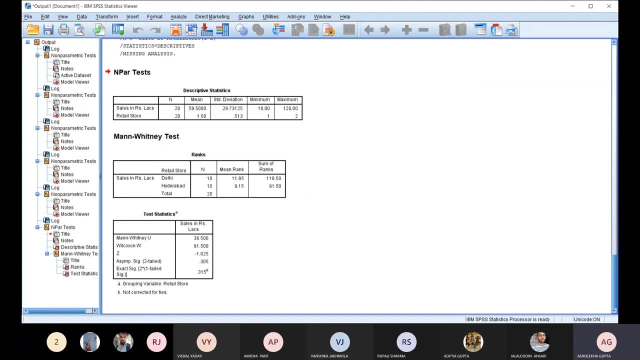 So objective is this that we have to customize automatically. we have defined the field here: right sales is visible. why? Because now what we have to do, what we have to do in our statistical file here, where we have defined the variable, if we take string retail store rather than numeric right. 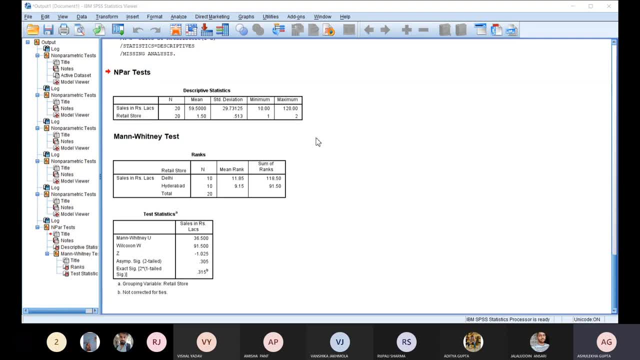 You have stringed right and after stringing what you have done, You have made it nominal here, right Now. you now we will run. now we will run. we went to analyze. after going to analyze, we have done non-parametric test and independent sample. 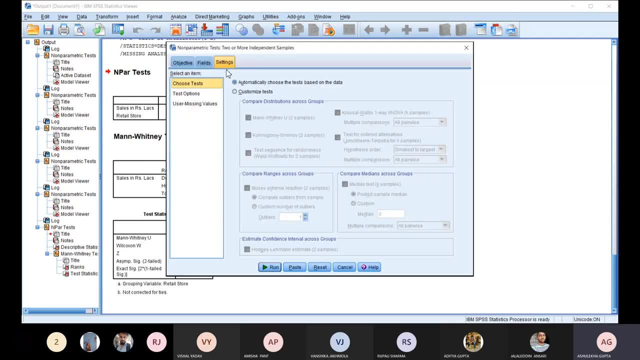 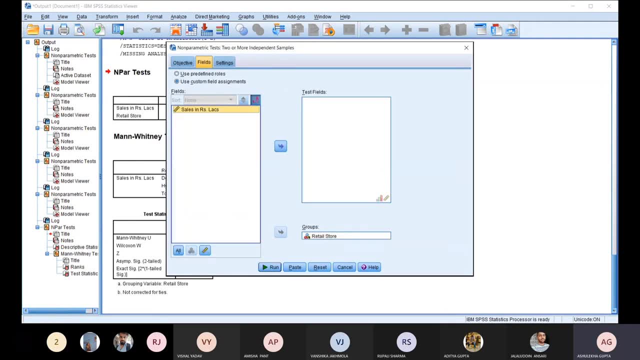 So if you look at objectives, then here automatically choose the test. right. we went to fields. we return it to fields. we have not saved it yet. right retail store is here. We have shifted the retail store to this side. Right. so now you see we have shifted the retail store to the group. we have put the test variable in this, right and now we will. and let's see in settings, in settings, automatically, right, so we have run it. so you see this. we have this table. 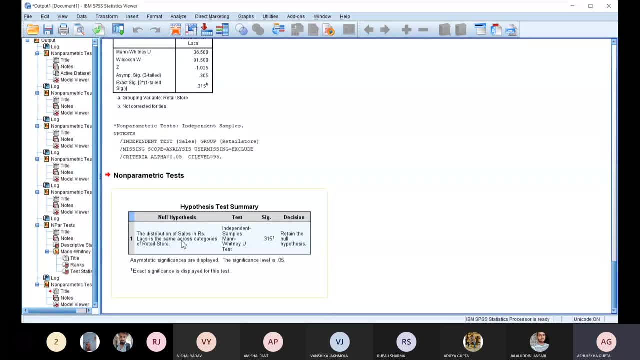 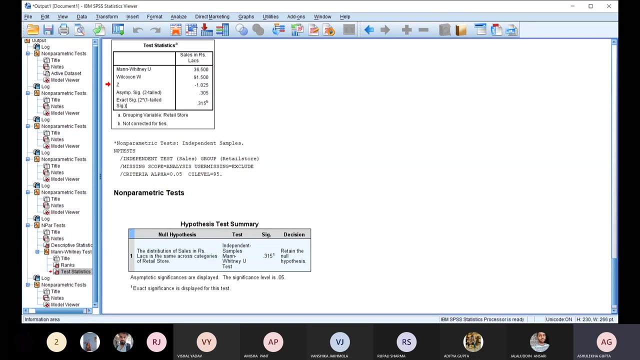 What is sure, the distribution of sales and rupees legs is the same across categories of retail store. So independent sample, it is not a new test. it is a new test significance level because point 0,, 5,, 6 is bigger. so we will retain the null hypothesis and we will reject alternate hypothesis and we will copy this table. and where will we take it? in our word document. right in the word document. and we will copy this table and we can carry forward to our word document, right. 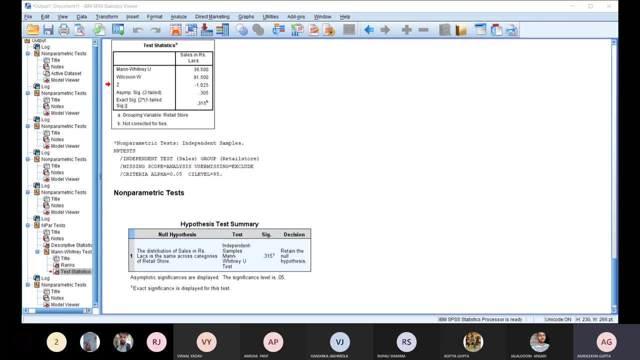 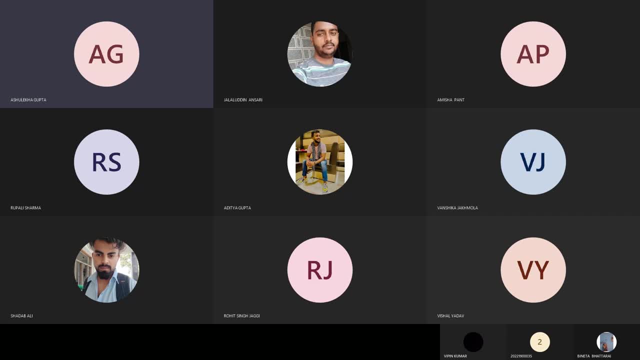 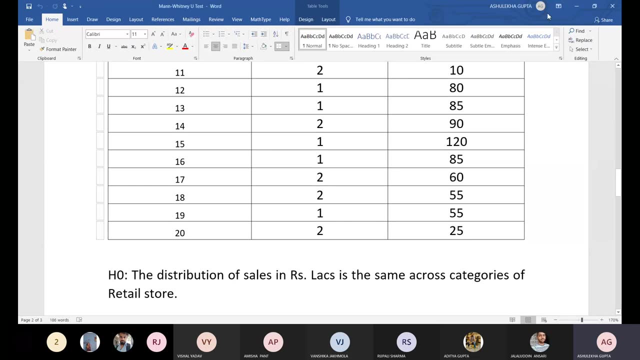 You could see I am sharing my screen word document. you could see here What document name. now again, right, Yeah, this is the we can see here. you table I'm are a part. This is the table, right. 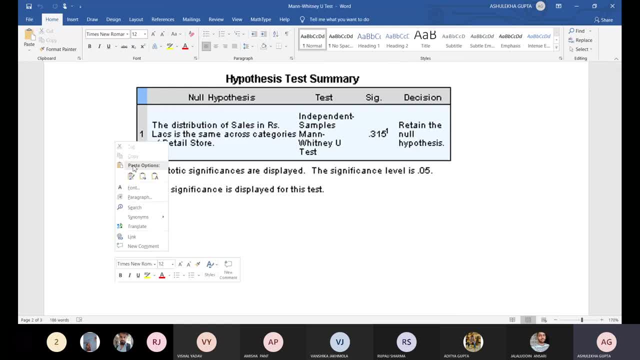 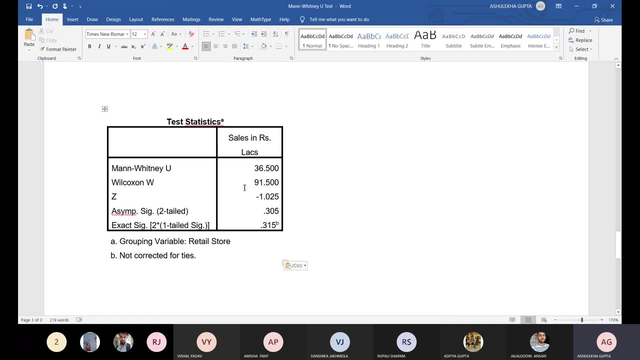 And another table also. we we are carrying this- Could be happy. how peaceful that they have stable go be right. These are the. yeah, we chose these And we can see that when you see this, This one, Okay, here, two independent variable may jacket, army, a table miller, again significant. 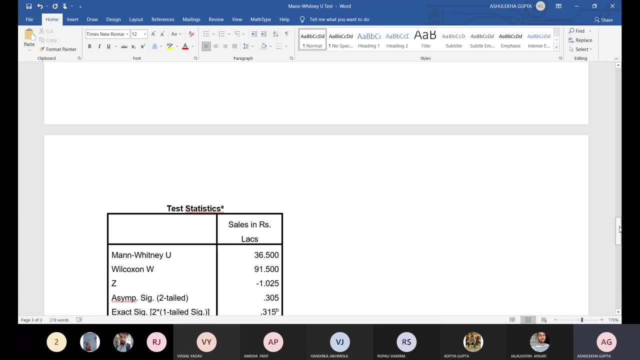 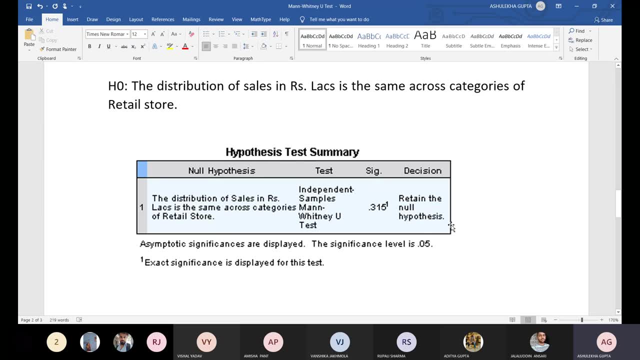 system, point three zero five right. and here is also point three one five. to retain carrying a home. null hypothesis for why we are retaining: because our p value is greater than point zero five. so that is why we will retain. this is our null hypothesis. is for home care. carrying a is for home, except carrying.